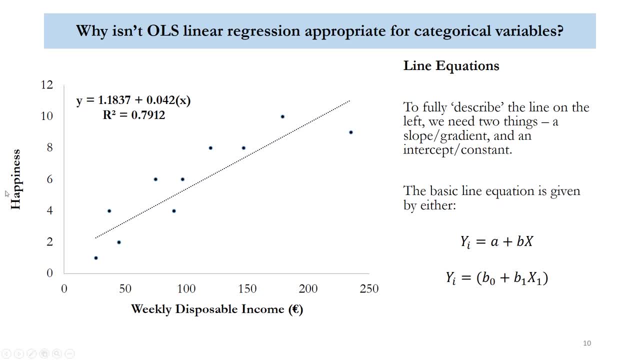 all invariably. so far, we've looked at the case of continuous dependent variables. In other words, what we've tried to do so far in the lab is to model dependent variables that are measured at the scale level, or approximately at the scale level. We've looked at a couple of a couple of 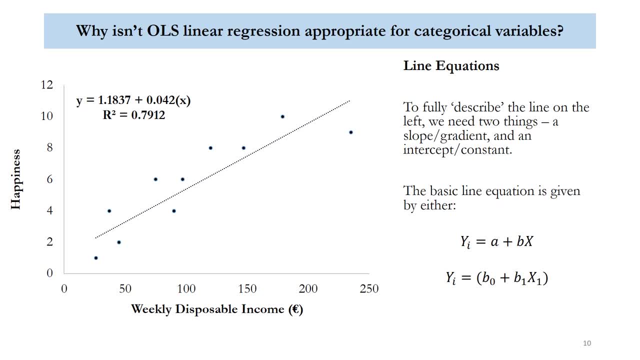 sort of pseudo-ordinal attitudinal measures so far, but in many different branches of the social sciences we do not deal with continuous outcomes. If you look at the contents of the ESS dataset, you'll notice that the majority of variables there are categorical variables. That's because in the 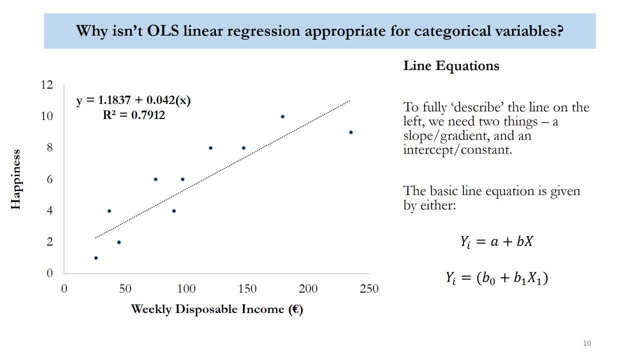 social sciences. all the time we deal with things that vary in terms of categories. We deal with different ratios, groups, different class groups. We also deal with things that can't neatly be allocated to a continuous measure, Things like attitudes or membership of a particular job or status or 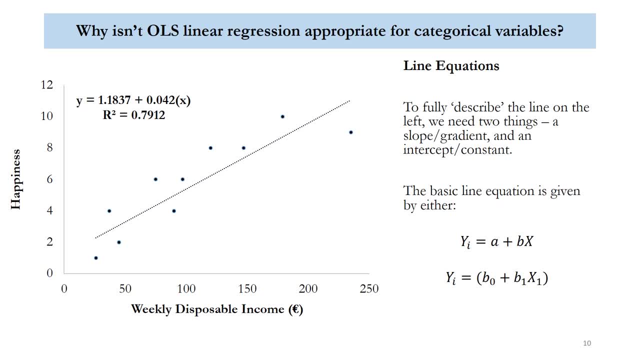 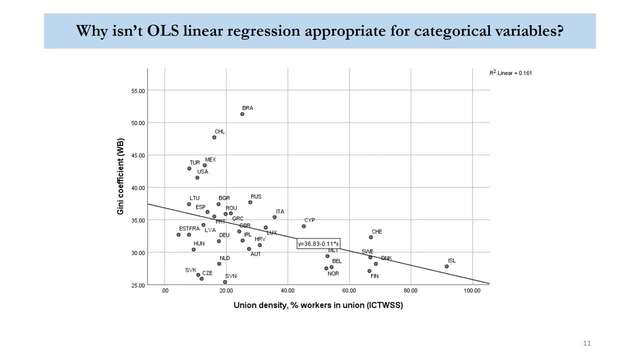 whether or not somebody does something like whether they vote or not, or whether they vote for a particular party. So to address this, we need a different family of techniques, and the method that we're going to look at in this course for the final week is the method of binary logistic regression. So, as we've seen so far, 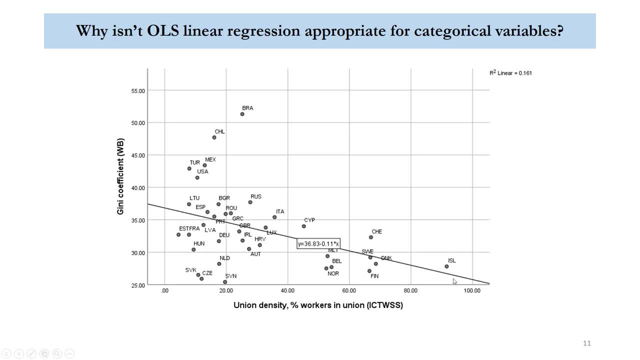 the cases that we've been dealing with. if we look at the teaching example that we have used for the last two weeks, we can approximate the relationship between two continuous variables, in this case union density and inequality, with a linear fit. We fit this linear line through our data points. 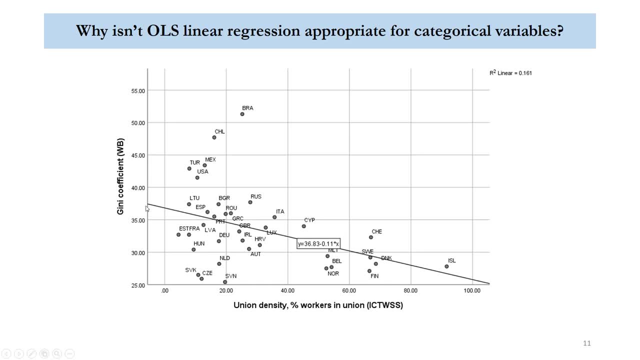 here and we get a prediction equation with an intercept and a slope. This shows us that for each additional percentage point of union density at the country level, there is a corresponding decrease in average inequality amongst our country set of 0.11 units In this. 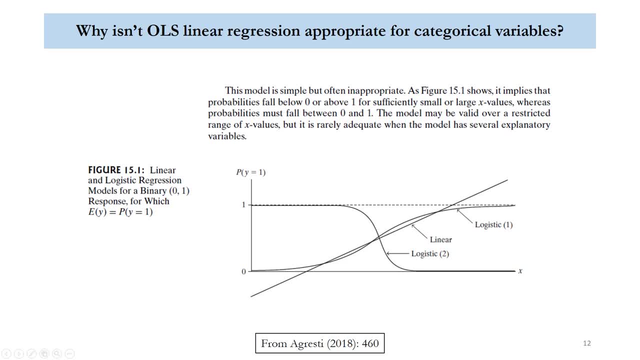 case, this is Gini units, But we run into a problem when we try to deal with a variable that is measured in a different way, And the type of variable that we're going to look at now is what's called a binary categorical variable, And that's a variable that can either that generally. 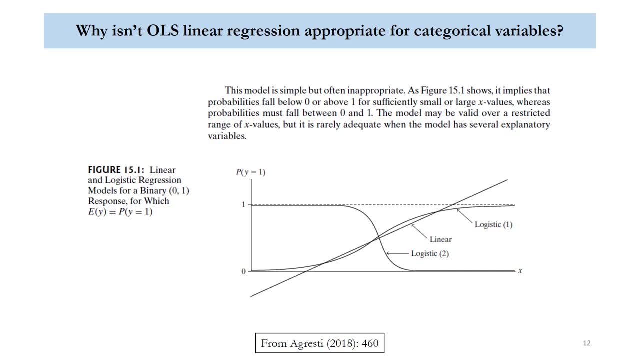 takes a value of 0, 1, 1, 2.. I'm going to suggest later on that we stick to the 0, 1 coding, just to make things easier. But we have a problem here, which is where, if we look at, if we have a, 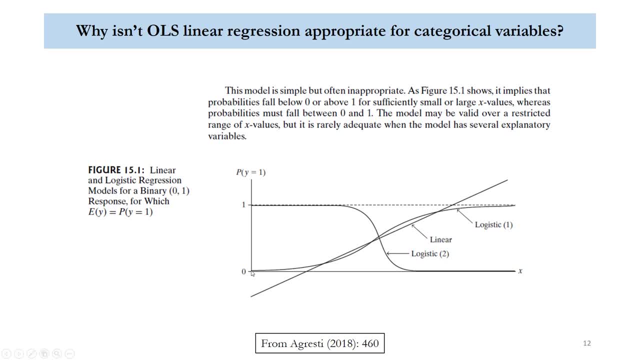 variable- let's say we have the example we're going to look at soon- is the vote variable. So whether somebody votes doesn't vote, or whether they do vote, And if you remember back to your SPSS coding, the way that variable is set up is 0- identifies someone who didn't vote- and 1. 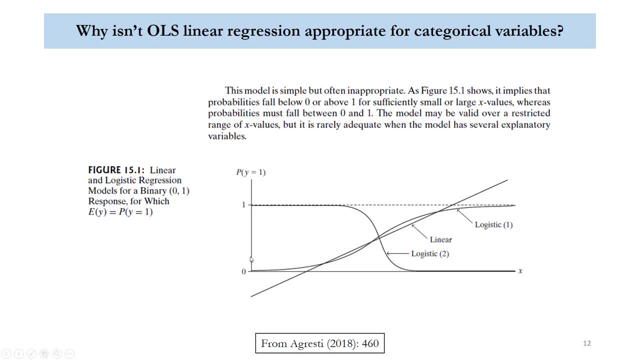 identifies someone who did vote, So that variable is coded 0, 1.. And if we tried to fit a linear model to that we would run into a problem. So we're going to look at a variable that is run into a problem And this is a problem. that's general to what we call bounded variables, like 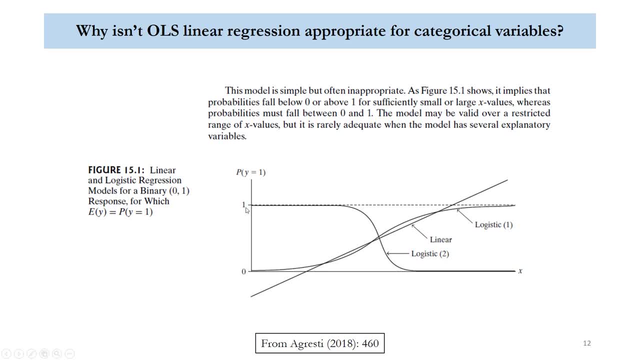 this. Somebody can either be in the state or out of the state. They can have voted, they can have not voted. But the problem here is that when we fit a linear model to this, we see that we have this problem where our model can in theory predict below 0 and above 1.. And we also have a 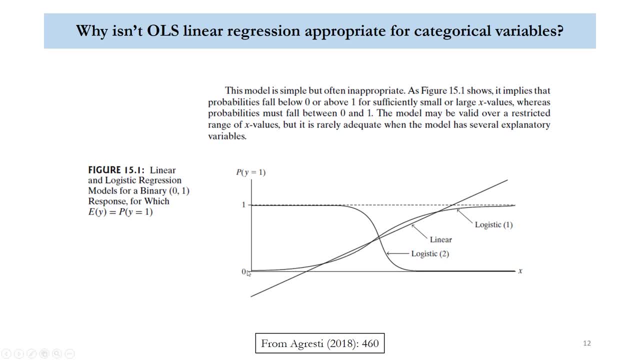 problem, which is that the change in the odds of voting from this sort of completely out to completely in state is nonlinear. We see that it actually approximates what's known as a logistic function. So the odds as we move from 0 to 1, the probability of voting, not voting, does not vary in a linear function, And this is an 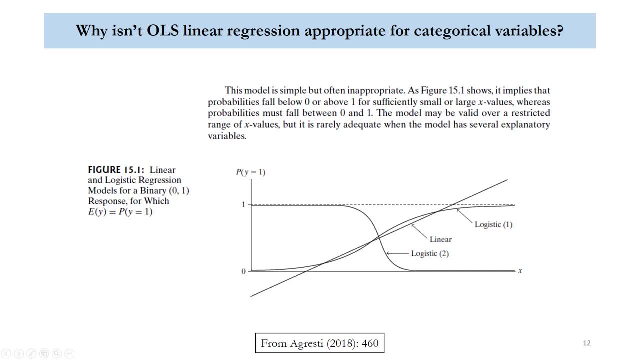 assumption, The linear assumption, is one that we could have relied on previously in the case of ordinary least squares regression, And we saw last week how we could diagnose our model to see if it met those assumptions of linearity, if indeed the linear model was valid. 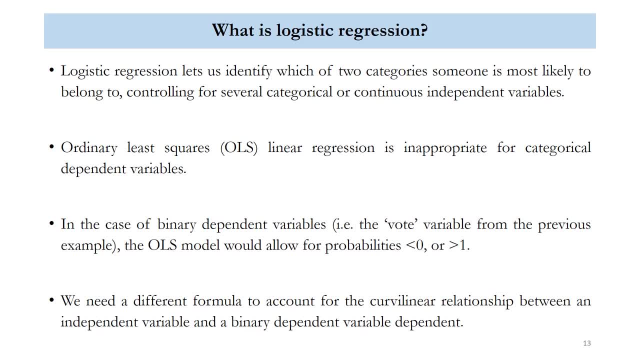 So we're going to look at a family of techniques to account for this. The one that we're going to look at is logistic regression. So logistic regression allows us to identify which of two categories- again remember, we're dealing with categorical variables- generally nominal variables or sometimes recoded ordinal. 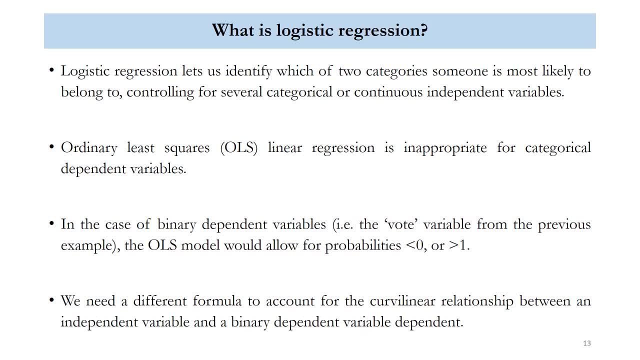 variables, And it allows us to identify which of two categories someone is most likely to be to belong to. we're going to talk about this in a number of respects. we'll use the term success or failure later on And like regression again. the nice thing about this is a lot of this. we can interpret the. 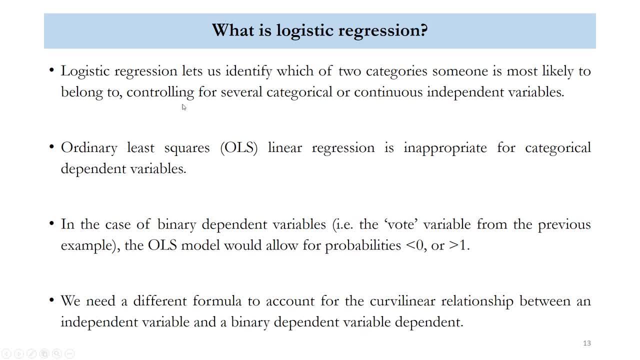 output of these models in terms of what we looked at already. we can also control for several categorical or continuous independent variables. So in the example that we're going to look at soon, we're going to try and model whether or not someone votes, but we're going to look at several additional. 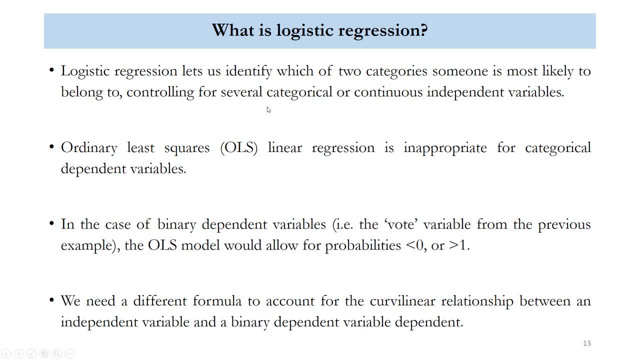 control variables or independent variables. So we're going to look at education, political activity, and we'll look at one other. So the ordinary least squares linear regression model is typically inappropriate for categorical dependent variables for the reasons that we've seen here. 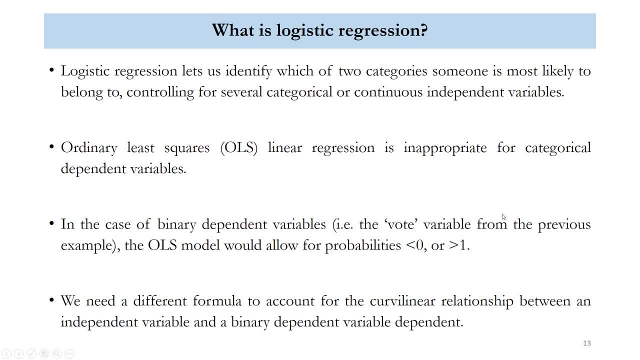 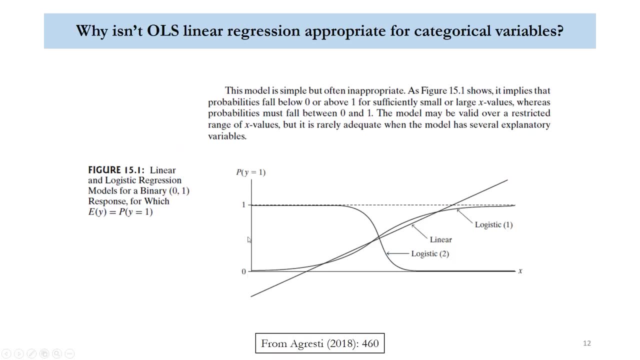 In the case of binary variables, for example the vote variable from the previous example in the previous slide, the problem here is that, as we saw, the OLS model will allow for probabilities less than zero or greater than one, which in reality is untenable because, given the way that these are coded and given the nature of the variable itself, we can only have a condition that goes from either zero or one. someone can either do something, experience an outcome, or they can not do something. 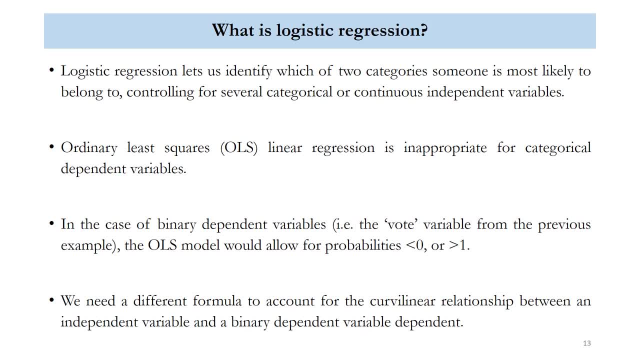 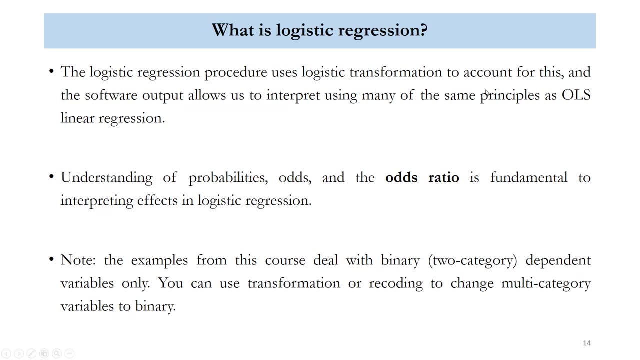 So we need a different formula, So we need a different model or different modeling approach to account for this curvilinear relationship between an independent variable and a binary dependent variable. So the logistic regression procedure is one that uses what's called the logistic transformation to account for this. 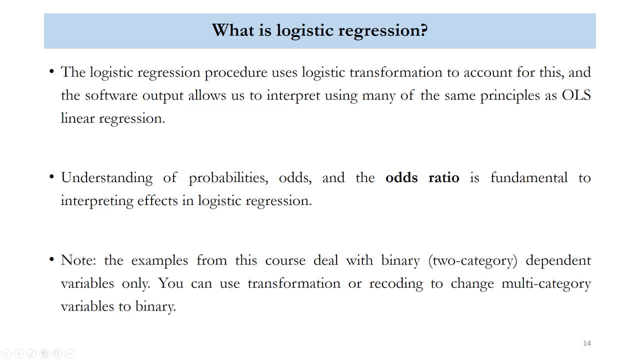 And the nice thing about the examples that we're going to look at for the remainder of this course, for week 12, are that we can interpret these in terms of some of the same principles that we use with OLS, linear regression. So we will look at effects, We will look at coefficients, We will also look at inferences. 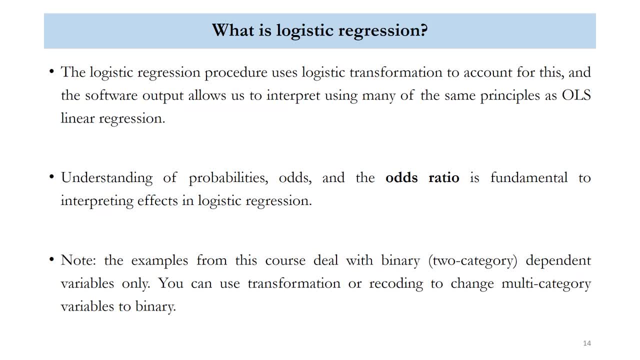 We will calculate p-values for those and we will also look at overall summaries of the model, like the R squared. we can Approximate that in a logistic regression context as well, to see how well our model fits the data. Now, to understand how logistic regression works, We need to understand a couple of key terms, and these are not too difficult to understand. 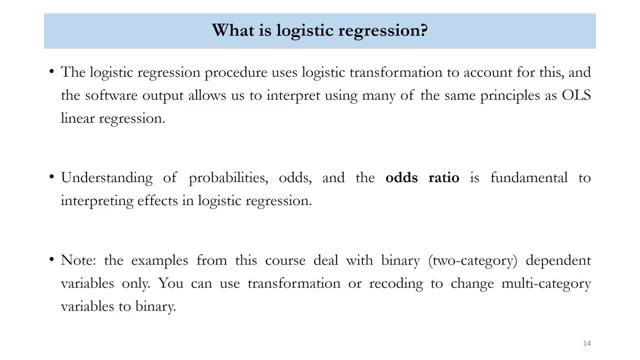 We can, the prop, we can get a good handle on these with just some simple division and multiplication. So we need to understand probabilities, odds and then, stemming from that, the odds ratio, Which is fundamental to interpreting effects in logistic regression. So the examples that we will deal with in this course deal with the binary case. 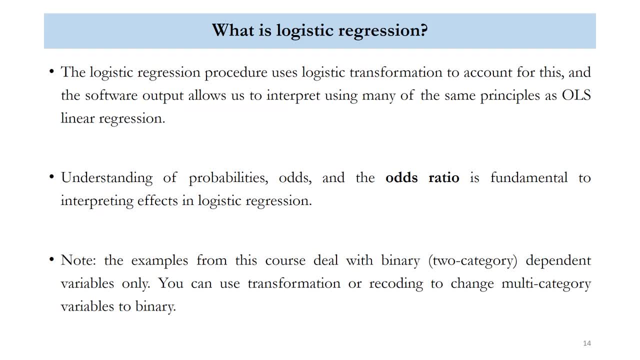 Which is a dependent variable with two categories. So somebody voted, somebody didn't, somebody smoke, somebody doesn't. in practice, you can Take this, you can extend this further in two ways. There are techniques that build on this that can deal with multi category dependent variables, but I'll also show you, if you wish, how you can transform existing multi category variables into two category variables. an: 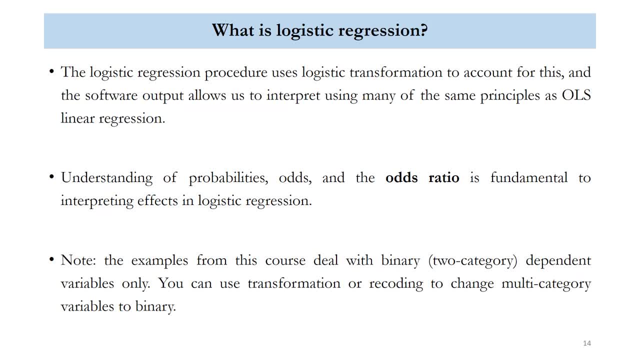 Example here would be: if you had a party voting variable, if you wanted to model people that just voted for one party, Let's say Fianna Fáil- But you had a variable that measured whether somebody voted for several different parties, Then you can recode that variable to identify just the people who voted for one particular party. 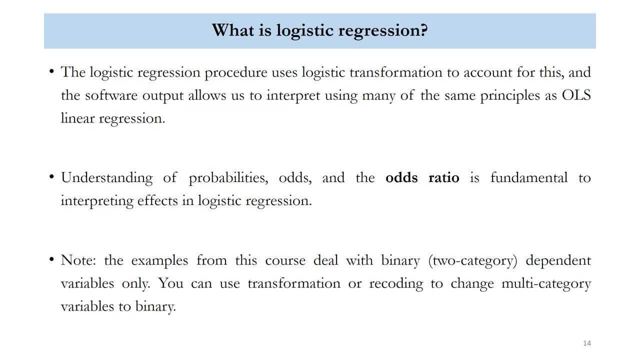 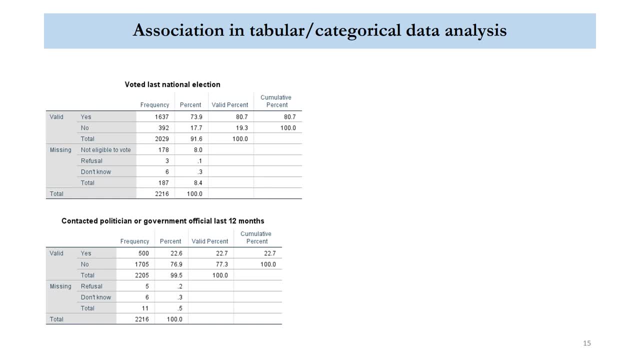 And this recoding is a useful application that you might come back to for future projects. So let's have a look and see how we would Characterize association, first of all in a tabular, categorical data context. So I'm going to demonstrate the calculation of the odds and the odds ratio here. 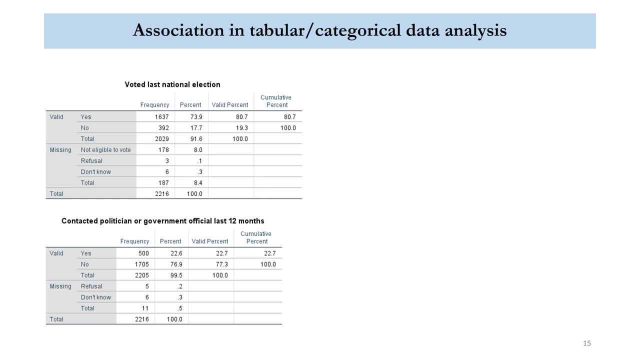 And then we will apply this to an example using some SPSS output from a binary logistic regression. So here we have two variables, We have what's going to be our dependent variable, Which is whether or not the people, whether whether or not the respondent, voted in the last national election. and in this sample we see: 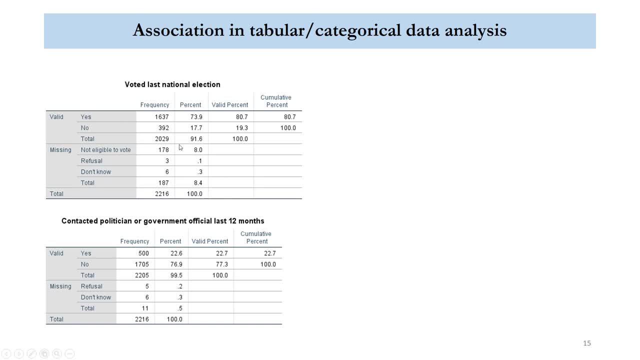 Here we've got two thousand two hundred and sixteen respondents, 2029 valid cases. eighty point seven percent of those did vote and nineteen point three percent didn't. And if we were trying to explain why somebody would or would not have voted, we could look at several different factors. 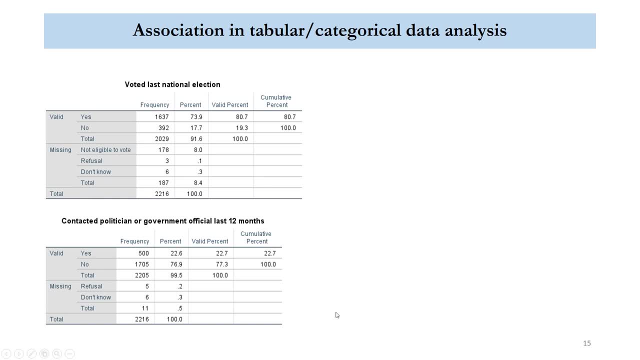 But in this one we will look at a proxy measure of political engagement. We will take as an indicator that someone is political engaged, whether they say yes or no to this question. So this question asks: have you contacted a politician or government official in the last 12 months? 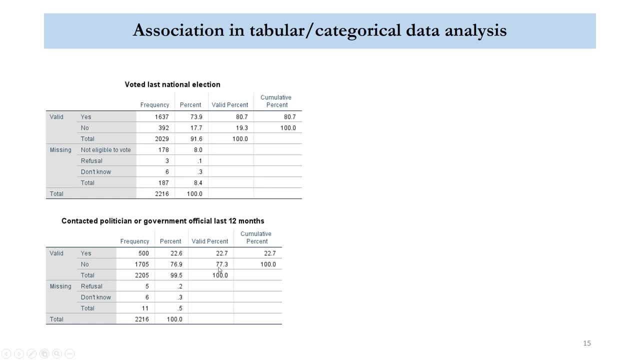 And of the valid sample, twenty two point seven percent did and seventy seven point three percent did not. So we could express this a different way if we took this, This table here, if we just take the vote variable. first of all, here We have a case of a binary categorical variable. 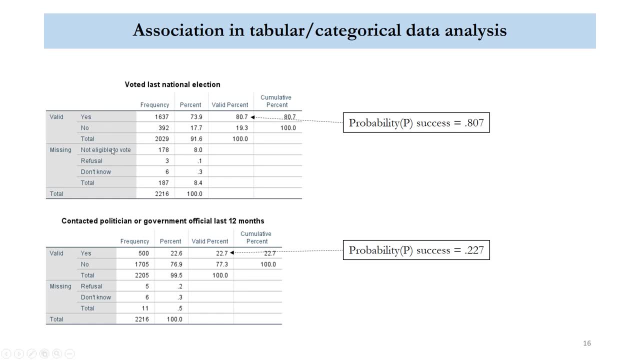 It's binary because it's got two possible options: Yes or no. You see we've coded. the other categories here is missing, So they don't count and they don't count in the final variable and we could transform this to say that we could Approximate the probability of somebody voting. by transforming this: we simply multiply this out by one. 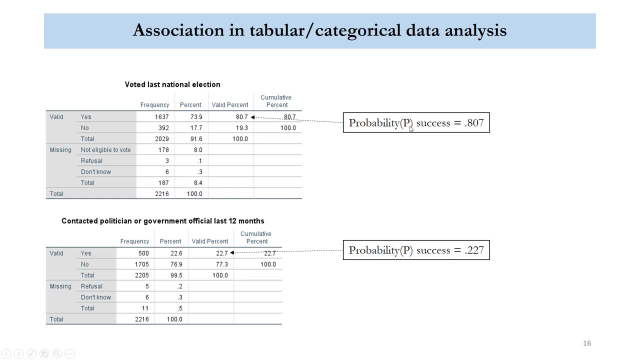 So I divide this by a hundred and we got a probability of success or a probability of having voted of point eight, zero, seven. In the second case, the probability of someone having contacted a politician or government official is point two to seven. again, using this transformation from percentages to proportions, 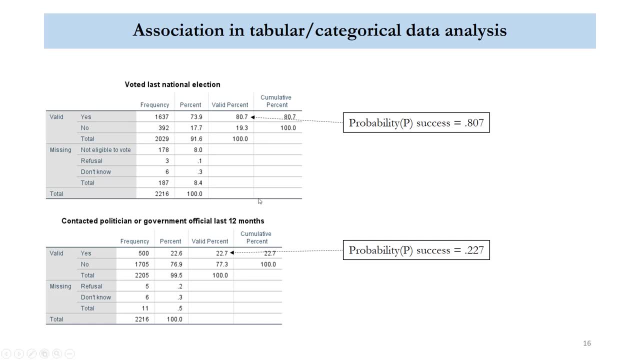 So in the first instance we can transform both of these, both of these properties, here, the, The percentages, to probabilities and we can express this as a probability of success- point eight, zero, seven- or a probability of failure- Point one, nine, three. So you'll see in the literature, quite often in the textbooks for this and when they're explaining logistic regression effects and odds ratios, 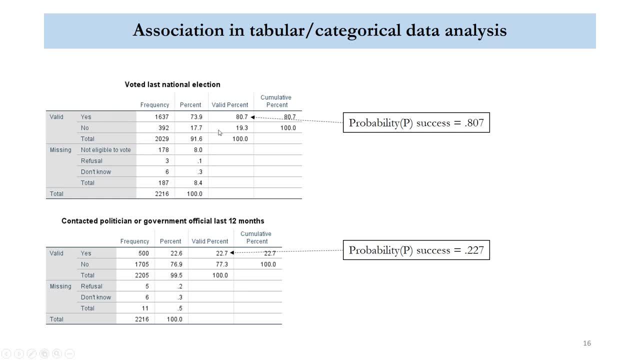 They'll talk about success and failure And generally you can sort of interpret these as the yes-no categories. So here's the general rule that we follow. we can convert percentages to proportions, in this case by dividing by a hundred. You'll see, here We've got twenty two, point seven, and this becomes point two, two seven. 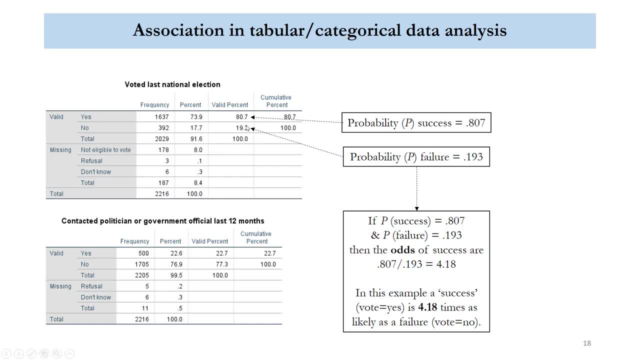 So, stemming from this, then for any of these and again we'll take these tables on isolation. first of all, We'll just start with the vote table. if the probability of success then in this table is point eight, zero, seven, success being a voter, Yes, and the probability of failure is point one, nine, three. 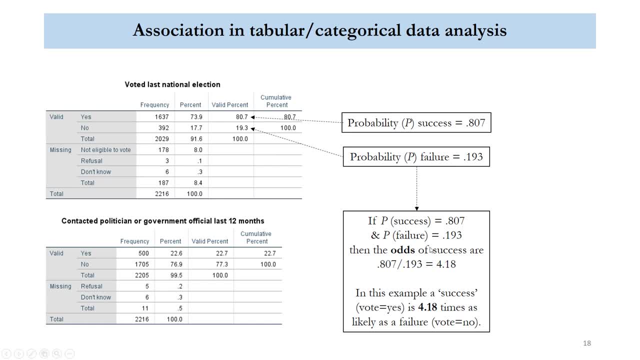 Then we can calculate the odds of voting, and the odds in this case are simply the probability of success divided by the probability of failure, Which gives us a figure of four point one eight. So these are the odds of voting, These are the odds of having voted. So, in this example, a success, a vote, the odds of having a vote. 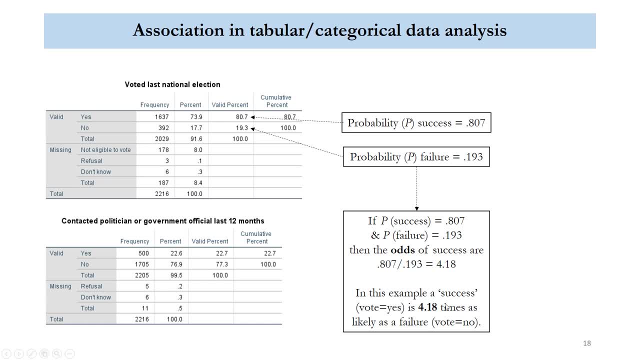 Are four point one times as likely as a failure. So this probabilities and the ratio of success to failure is four point one, eight times As likely as a failure. in this case, vote equals no. So let's look at this now in a two by two context. 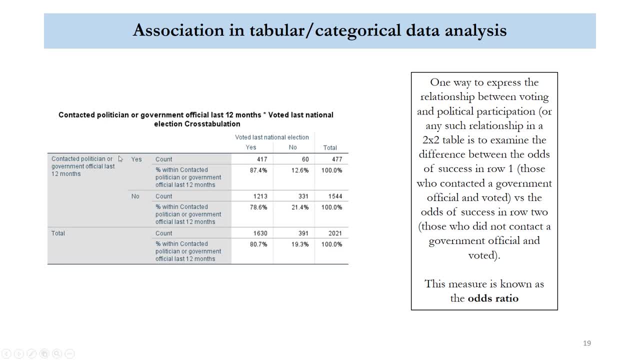 So when we combine these two variables together In a contingency table, we get a table, a row by column table, Which shows us the percentages or the proportions of individuals who have contacted the politician who voted and the proportions of individuals who did not contact the politician who voted, and we see a little difference here. we can see that. 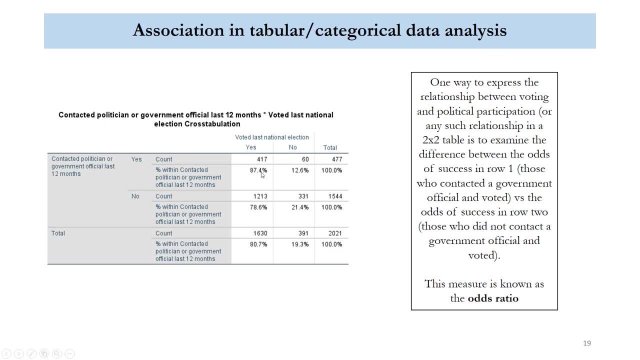 Respondents who did contact a politician, ie are more politically engaged, are also more likely to have voted. Eighty seven point four percent of those who contacted a politician voted, relative to seventy eight point six percent of those who did not. now, a more Precise way to express this relationship, and again one that doesn't rely as much on on the units in this case, is: 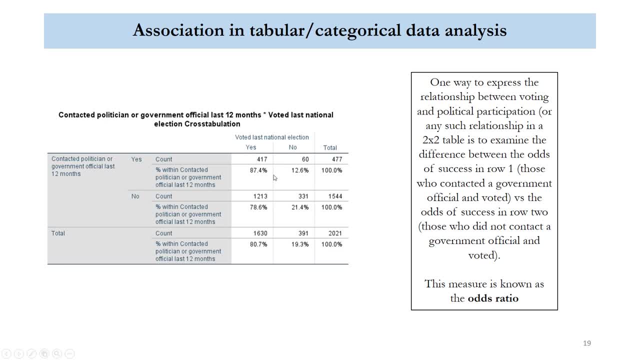 To examine the difference between the odds of success in the first row of this table Relative to the odds of success in the second row. in other words, What is the ratio of the odds of having voted Amongst people who do contact a politician relative to those who did not contact a politician? 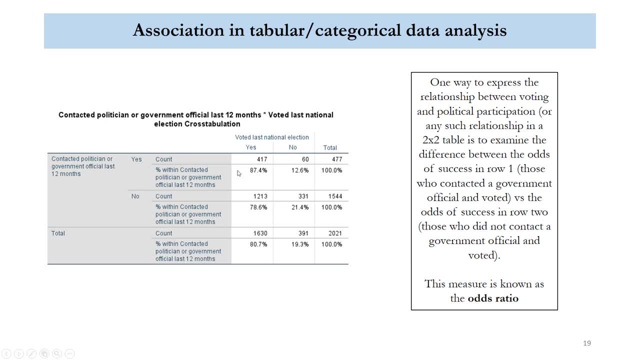 So this measure, this comparison of the odds of success and the first row relative to the second row, is what's known as the odds Ratio. so we're going to come up with a summary that allows us to express how much more likely someone is to have voted. 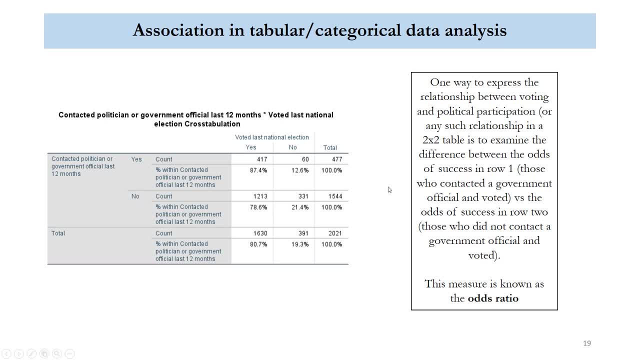 Given that they contacted a politician. and in these examples, in the example of the odds ratio, We're dealing exclusively with a two by two table, That's where we have two categories in the dependent and two categories in the independent. So, yes, no for both and yes, no for contact. 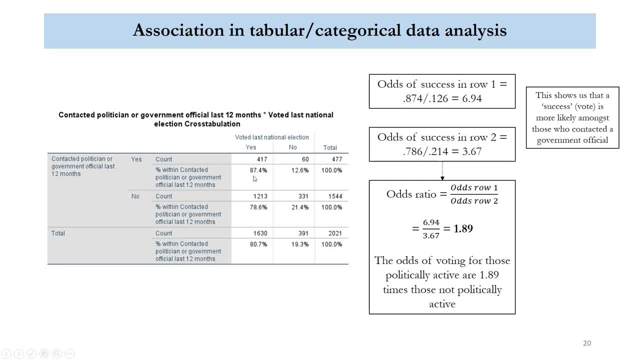 and To do this we simply divide the odds of the first row- odds of success in the first row- by the odds of success in the Second row, and we calculate that using the same procedure that we saw before. The odds of success in the first row, then, are point 8, 7, 4 divided by point 1, 2, 6. 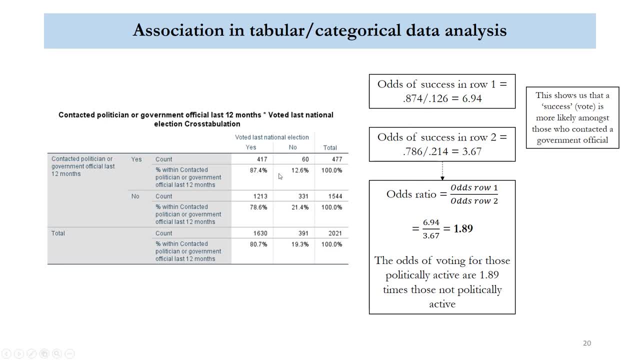 How do we get those two figures we divided by 100? We converted these two proportions. so our point 1, 2, 6 is simply a conversion of this twelve point six percent here. So we see that those who have contacted the politician, The ratio of success to failure, no to yes at six, point nine four: 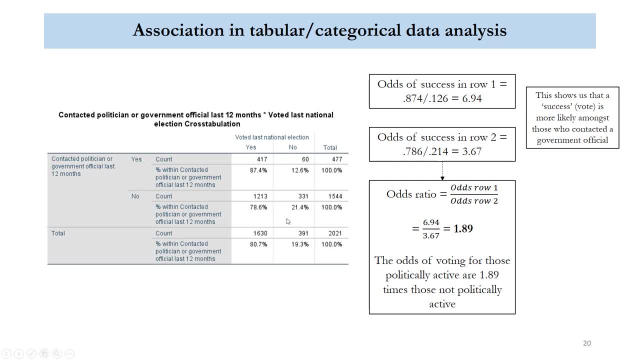 the odds of success in row two, then, are 0.214, sorry, 0.76, 0.786 over 0.214, and we get an odds ratio of 3.67. so we see here that the ratio of success to failure is higher in row one than it. 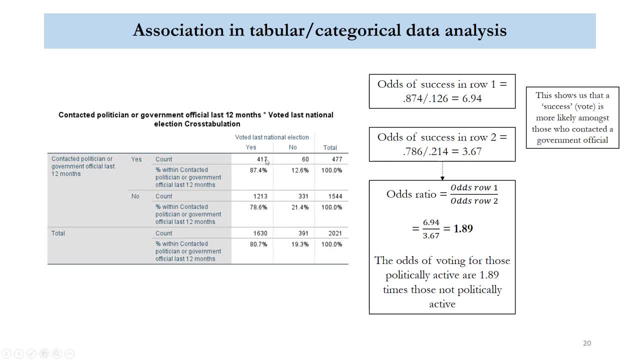 is in row two, but now we need to express this in terms of a comparison between this row and this row, in other words, the ratio of odds. how much more likely is it that someone will have voted, given that they did contact the politician, relative to those who didn't? so we simply divide the odds for 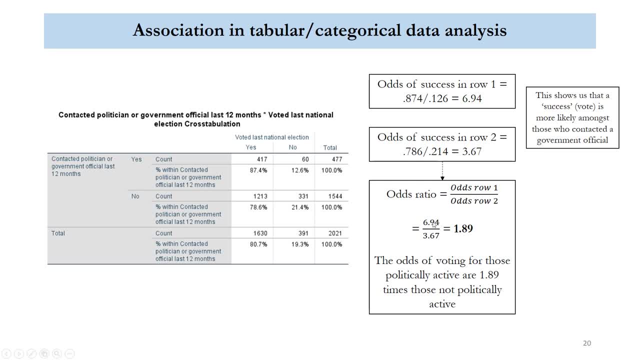 row one by the odds for row two. in this case it's 6.94, which is the row one odds over 3.67, the row two odds, and we get a figure here of 1.89. this is our odds ratio and the odds now of voting for. 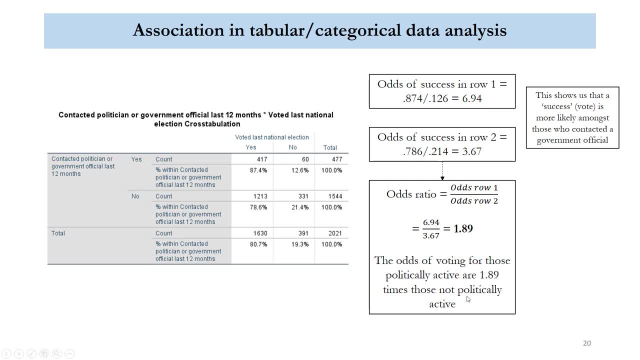 those politically active are 1.89 times those not politically active, and this allows us to summarize the relationship between these two variables in this two by two case that the odds of having voted for those who did contact the politician relative to those who didn't are 1.89, in other words, 1.89 times those who did contact relative. 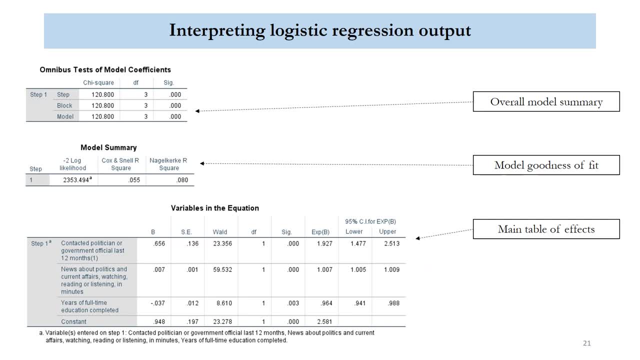 to those who did not now i'll talk you through the logistic regression procedure in the class and there'll be a short video available on youtube as well, talking you through the, the setup and the variable entry procedure. but we're going to focus in on three parts of output that are analogous to: 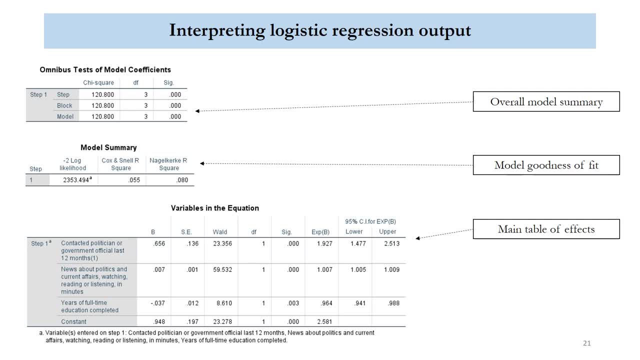 the ones that we've looked at so far in an ordinary least squares context, using continuous dependent variables. when we run the regression in spss, we can- we can get some of the same diagnostics that we looked at before. we can get residuals, we can get measures of influence, we can get our. 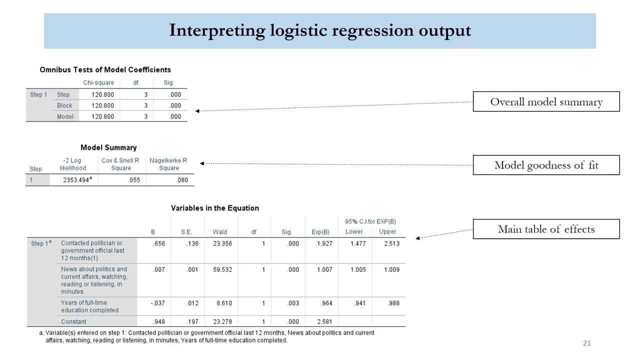 cook's distance and all that, and we can produce graphs and tables of those. but i'm going to focus in on the more important ones and the ones that allow us to assess, first of all, the overall model. the goodness there's, the overall significance of the model, the goodness of fit and the 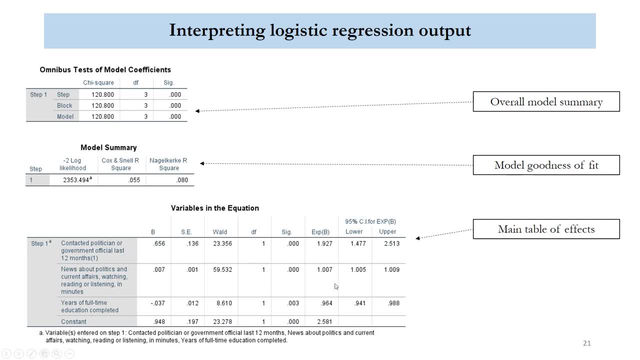 effectiveness of the model and then how to interpret the main effects, because this is what we're interested in really. down here is the main table of effects. what are the, what is the effect of each of these different variables? so, in this case, we have set up um, we have set up a model. 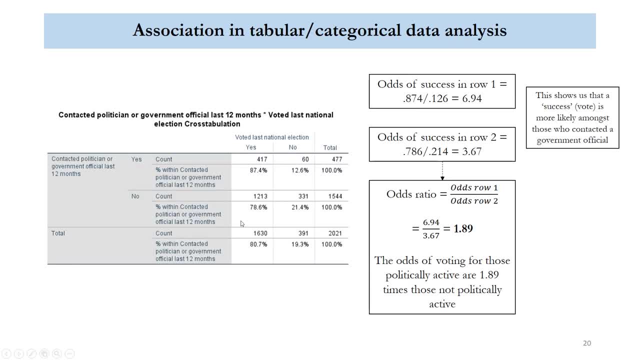 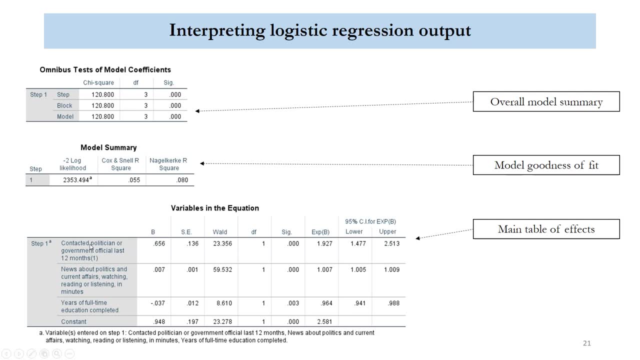 our dependent variable is the vote variable. it's this one here. it's whether or not somebody voted. our first independent variable, then, is the same as the one in the odds ratio example: it's whether or not someone contacted the politician or government official. and we also have two additional independent variables, or controls. we have this variable. 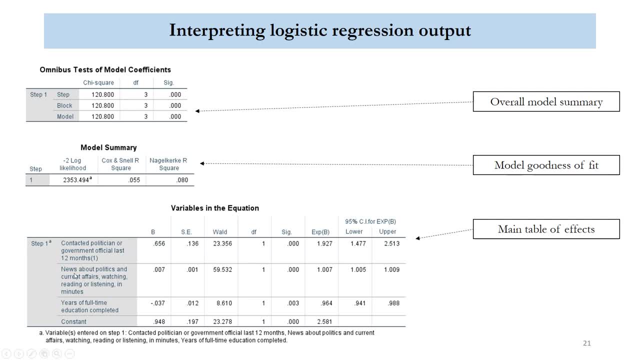 that asks people the number of minutes they spent, uh, consuming news about politics and current affairs, and this variable that measures years of full-time education completed. so how do we interpret each of these? the first table, then our omnibus tests of model coefficients, test the overall significance of the effects of our set of variables. so, again, this tested against the null. 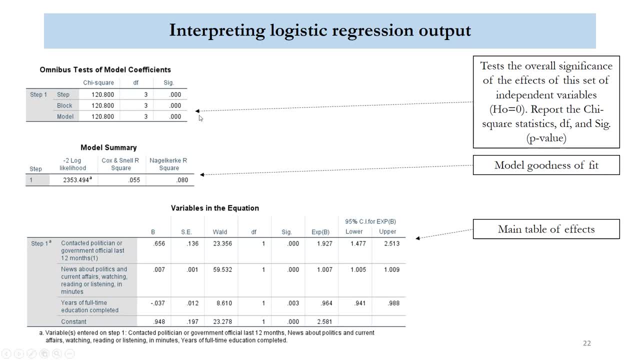 hypothesis that the effect of these variables combined is actually is actually zero. so again, testing this um, this, um, the this hypothesis that the cumulative effect of our variables is non-zero, in other words, that our variables are explaining, are explaining something, and in this case we see, spss gives us three. 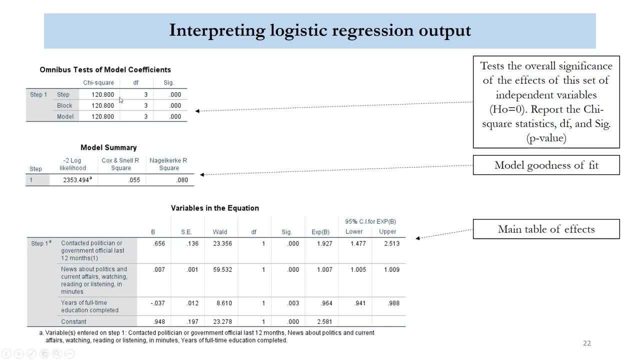 different ones. they're all the same here because basically there are. there are different ways that we can set this up. uh, we can use what's called stepwise entry or block entry, which is where we enter them in in groups and we we test the effects of different groups of variables, and block because 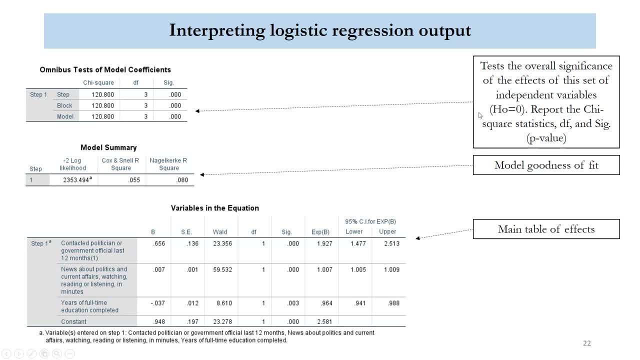 we don't didn't do this and we're not going to do this. these are all identical. so in this case, we will report the chi-square statistic, the df, which is the degrees of freedom, which in this case is equivalent to the number of independent variables- one, two, three- and the significance of our model. so here we have a. 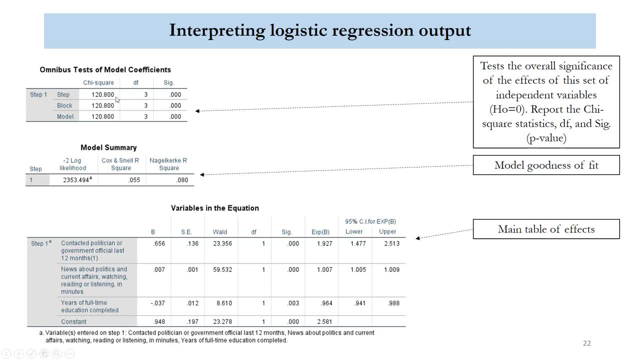 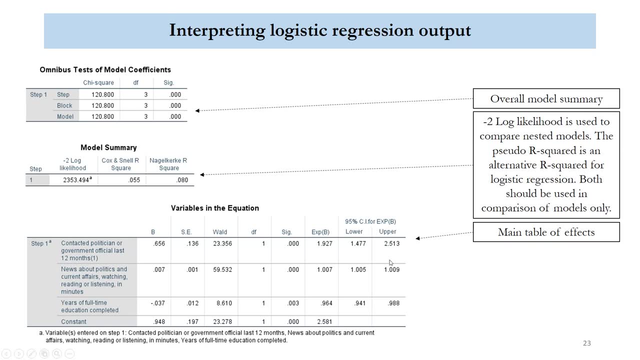 statistically significant model. our model is statistically significant relative to, relative to this null hypothesis. this ho equals zero model. the second indicator, then, is our model. goodness of fit, and we need to be cautious when we're interpreting this, because in the context of ols ordinary square's linear regression, we were able to interpret: 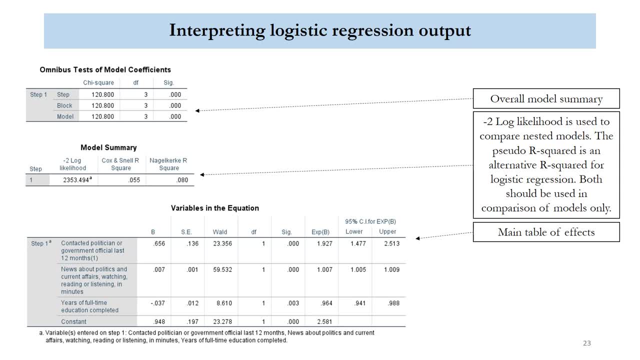 the r or squared, or our or our adjusted r squared, as the proportion of variance explained by our particular set of variables. um, these are what are often called pseudo r squareds. when you see these reported in the literature, they'll off. they'll always reference the type they use. but 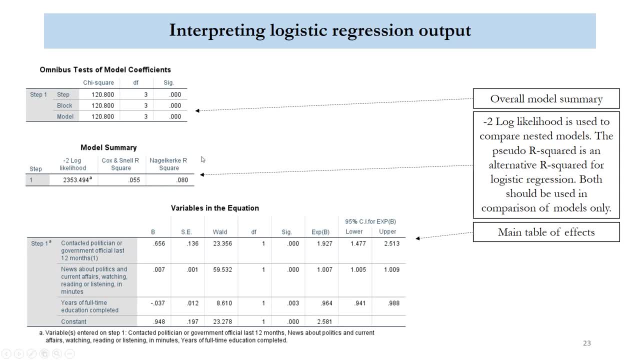 these are what's referred to as the pseudo r squared. it's an approximated r squared that's intended to do kind of the same thing in a logistic regression context. but these should not be used. these can't. these have no inherent meaning in and of themselves. these are only 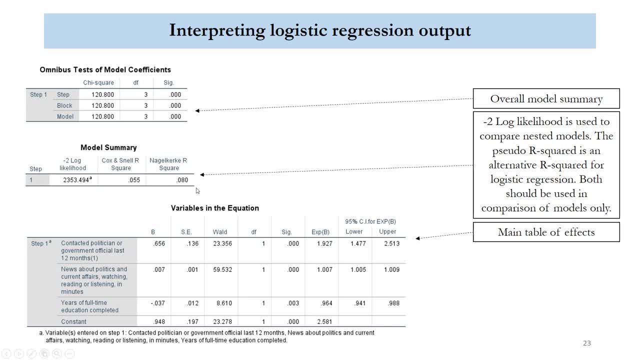 used in a logistic regression context to compare models. so if we had, let's say, a model with a specification like this that we wanted to compare against a more restricted specification, let's say one that just had one independent variable- this one here- then we would look at the comparison. 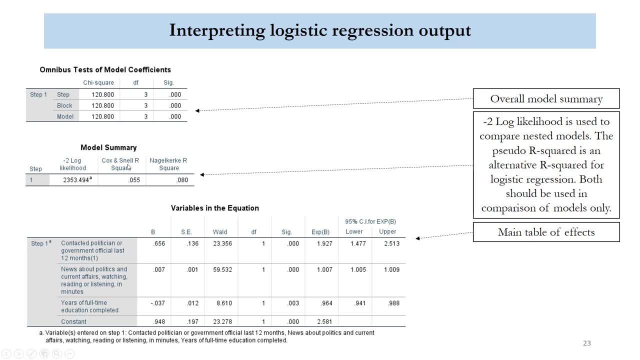 of either of our two pseudo or squareds. the one that we'll look at at the moment is the cox and snell critical model relative to the expanded model. so we certainly report these, but to and to really importantly use this in today's features, givenourd's perspective, when we take the billions of R squared that's the set of uh and we use that in instructively, that you know what users for using only three multiple powers- hence the but ones' arePreferred to רק er are Motoa and two more. You can use a few different types of standard variables, like super utilizzable, Limited in less than one variable can use a few decreasing 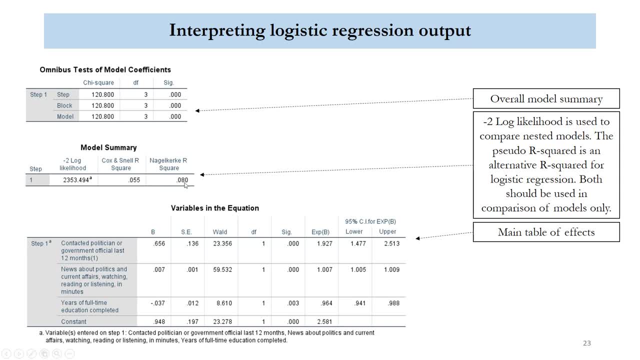 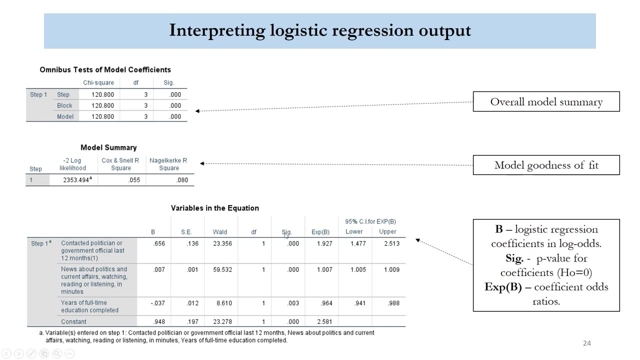 relative to the expanded model. so we certainly report these, but to interpret these, they have no inherent or intuitive interpretation. they can only be interpreted by comparison. now down here is our main table of effects, and we need to pay attention to a couple of things. we have three conditions here that we're going to look at, but in the reporting we'll look at a. 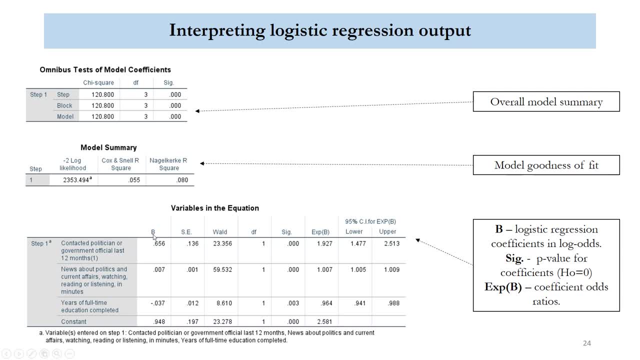 couple more the b column. then in spss these look a little bit different. in stata you have to add some additional options to get the table to. to return what, what? to return the? the different, the different figures that you want. so just be careful when you're reporting these in spss. the 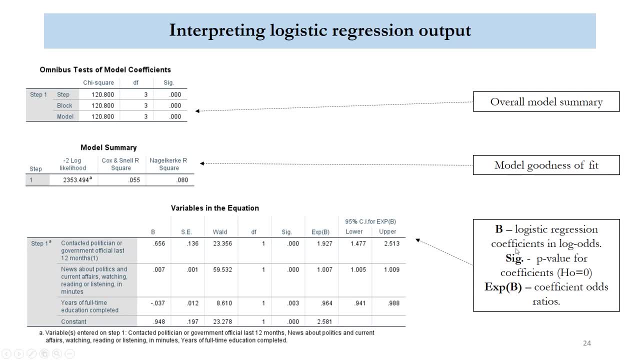 first column, with this capital b is the logistic regression coefficients in log odds. you'll often see these reported in the literature because these are essential to reconstruct what's called the prediction equation. if you remember back to our our first slide and if you want to wind it, 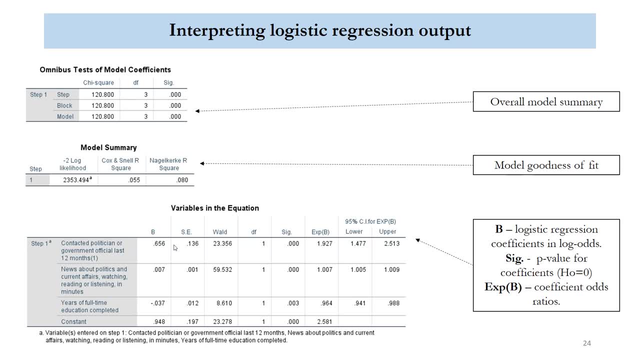 back to have a look. we had our our linear regression equation, um, presented on top of the scatter plot. now to reconstruct the equation, in other words um, to calculate the predicted probabilities given our sets of variables? you would need access to this information here. so this is important but um quite 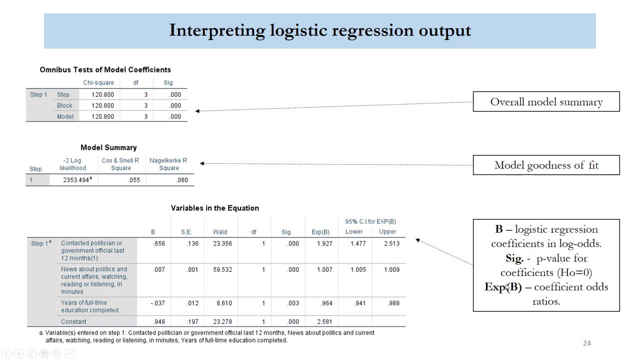 often you will see the odds ratios reported which are given over here in this exp brackets, capital b column, and these are the ones that we will focus on because, again, they make the effects a little bit easier to interpret and to compare across. so to fully reconstruct, if you like, the researchers original results, ie the 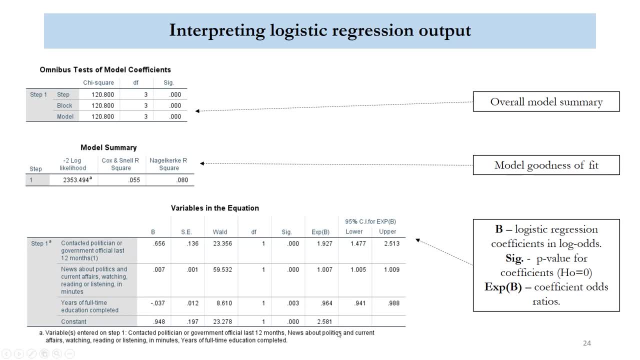 prediction equation. you would need these. these are important, but to interpret the effects and the effect size, these are also important as well. we also get a significance here, a p value, which is a test using the wall statistic. again, these are not t tests. um the test, the significance of our 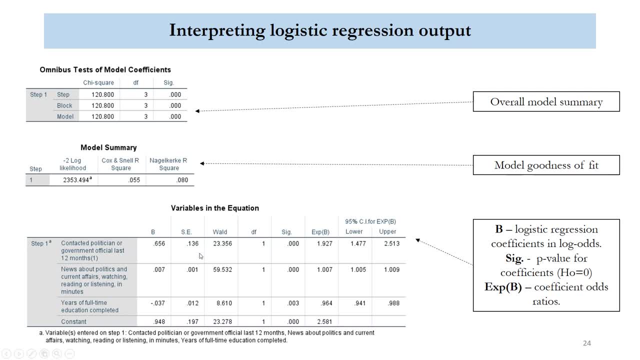 coefficient, again testing the effects of our slope or testing the individual value of our slope, and etc. so what we'll do is we'll be doing a fee, które study here and we'll be showing you, uh, the optimal success rates. it's up to us um to vida right now, so let's. 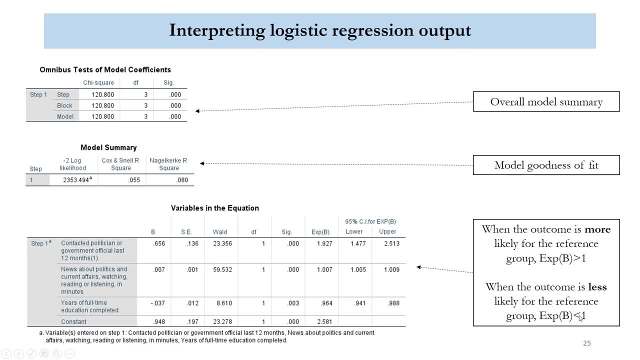 head off to look at this, but before some difference. when we look at these results in the will effect of this for the next example, we see here that the odds of voting for those who have contacted a politician are 1.927 times those who did not contact a politician. and again, this is controlling. 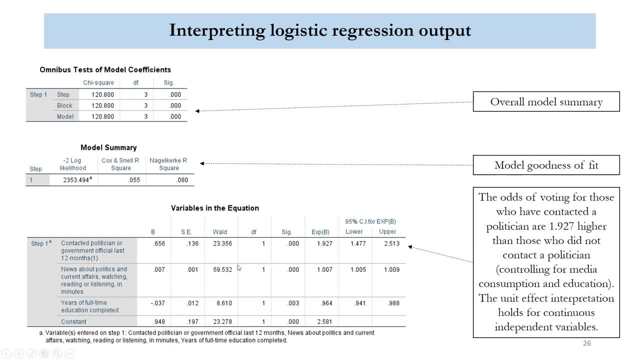 for media consumption and years of full-time education. remember, these are partial effects. this is controlling for the effects of the other included variables. what this actually means, then, is that the odds of having voted for those who did contact a politician are significantly higher. um sorry, the odds of having voted are significantly higher for those who have. 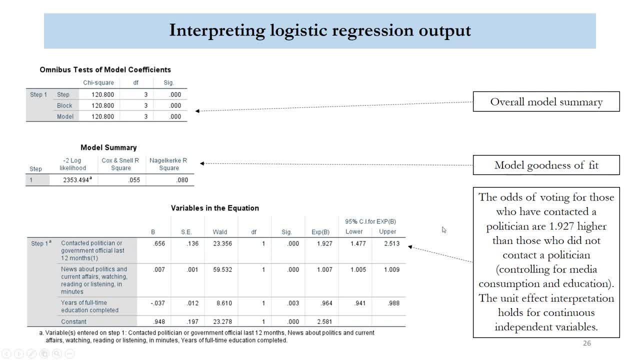 contacted the politician relative to those who did not. in this case, they're almost double. what you want to watch for when interpreting these effects first of all is whether or not the odds ratio passes one. if it's less than one, then it's less likely. you see, here this is quite 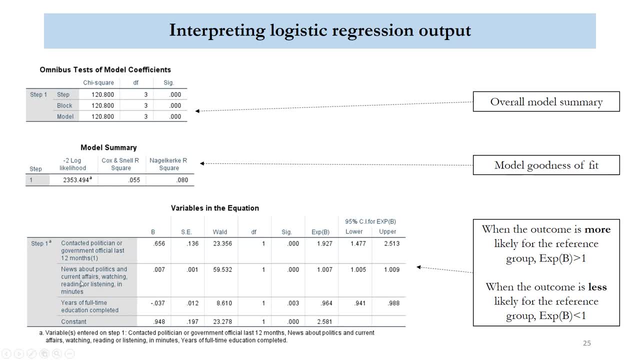 close to zero and again you've got to remember the units of this. this is for each additional minute of having watched news about current affairs. so again, we might want to perhaps transform this, maybe dividing it by um, dividing it by 60, to get the units and hours, or something this might make this. 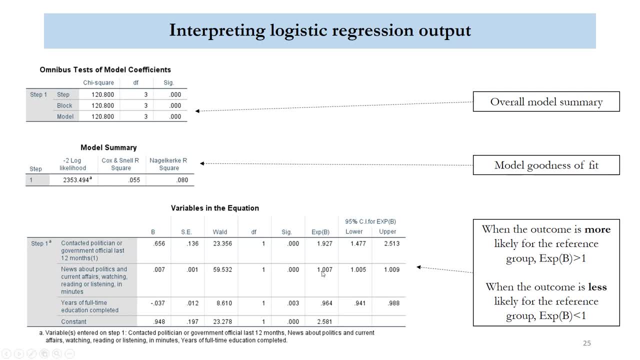 a bit easier to interpret. so the ratio of odds then, for those who consumed one additional minute of news media are 1.007 times those who did not consume that additional minute. similarly, for this one, this is a continuous variable that's measured in years of full-time education. and here we see: 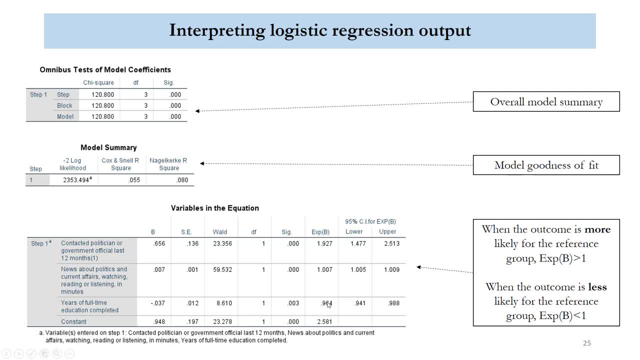 that, for each additional year, those with an additional year of education are marginally less likely to have voted, but these are the odds that we're going to be able to interpret. these are both quite small effects. as you can see here, this is quite a strong effect. 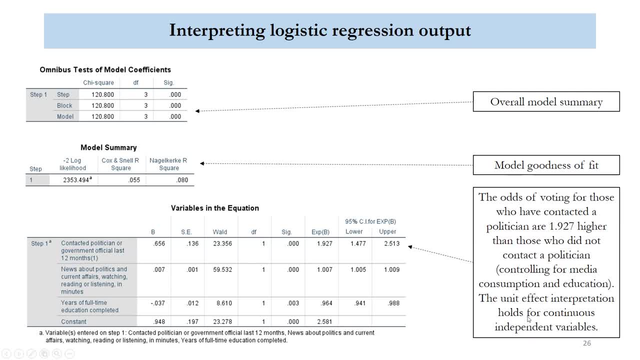 the unit effect interpretation holds for continuous independent variables. so, like i just said, this is the effect of each additional unit- in this case year, and the unit in this case being minutes. so you've got to be careful of the minutes when you're interpreting the effects of categorical. 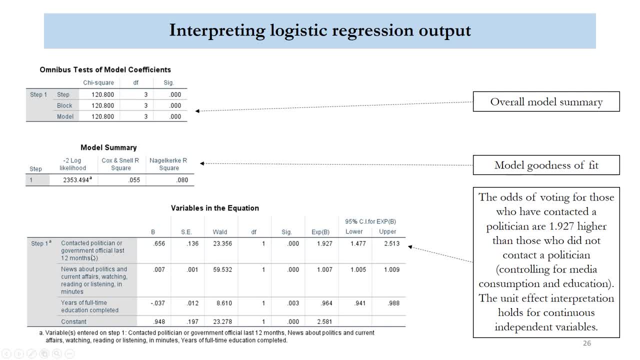 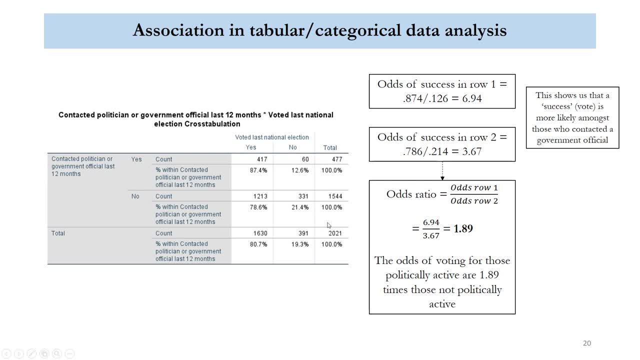 variables, in this case whether someone contacted a politician or government official in the last 12 months. we can revert to this interpretation here that we saw previously, which is that you can sort of visualize this as a two by two table with our yes, no, zero, one coded dependent. 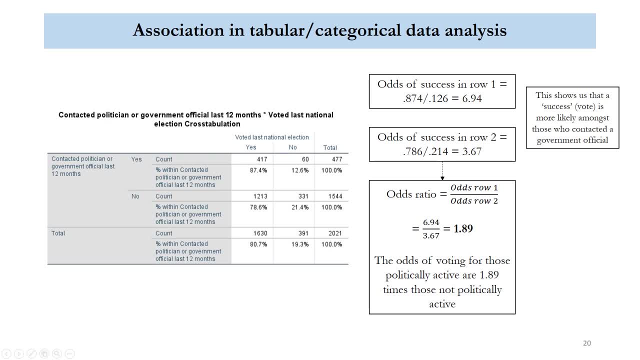 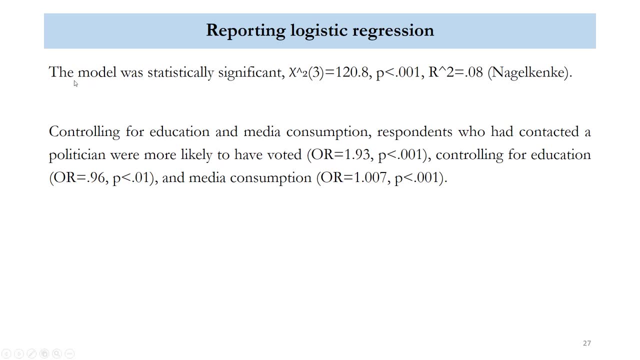 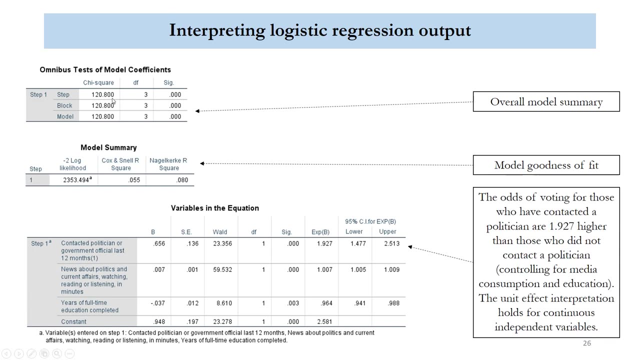 variable and our yes, no coded political contact variable. how you would report this, then, is you would say: first of all, the overall model summary, which is our model, was statistically significant. our chi squared figure, as we saw in the initial table, the model output was one, two, zero point. 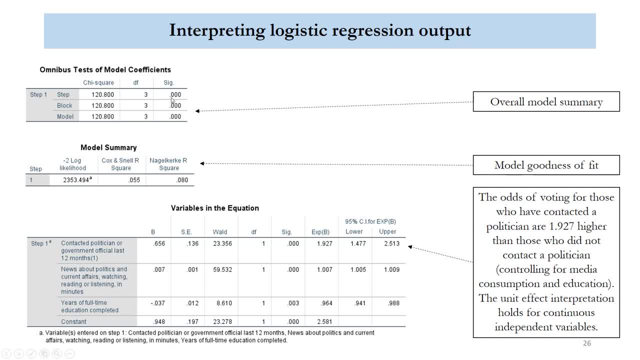 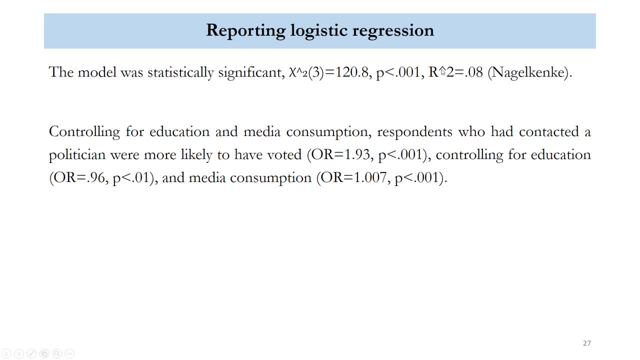 eight, with three degrees of freedom and a reported significance value of point zero, zero, zero. so we can say here that our value is, our model is statistically significant and our pseudo r squared, in this case in agilkenke, is 0.08. it's relatively small r squared, but again, we don't have that. 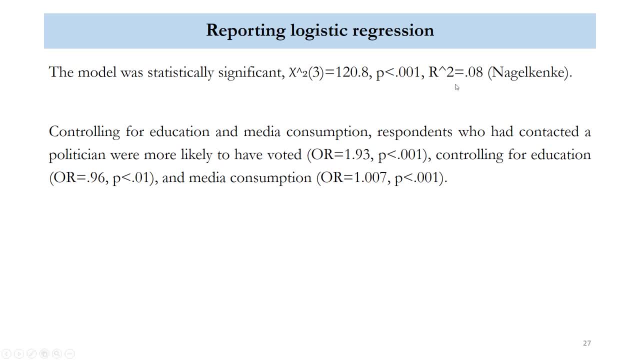 intuitive interpretation for this, like we did with the adjusted r squared in ordinary least squares regression context. if we were trying to describe the effects, then we would say that, controlling for education and media consumption, respondents who had contacted the politician were more likely to have voted. their odds ratio is 1.93. 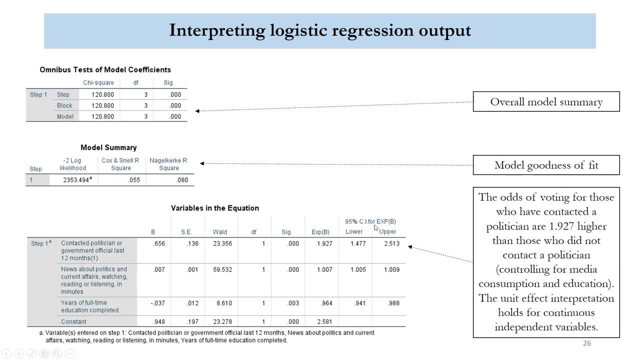 again remember it's important that we look as well at the 95 confidence interval. another: what's the likely range within which- because again, this is sample data, we're working with sample data- what is the range within which that's likely to have occurred? the confidence interval is quite 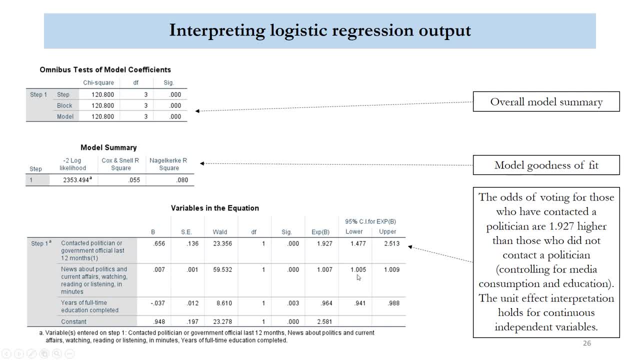 wide, as you can see here. what you do want to watch and see is if it crosses- if it crosses that one to less than one barrier, in which case we couldn't be entirely certain, or perhaps as confident, as confident as we'd like, that the effect was positive or negative in this case. these are all. 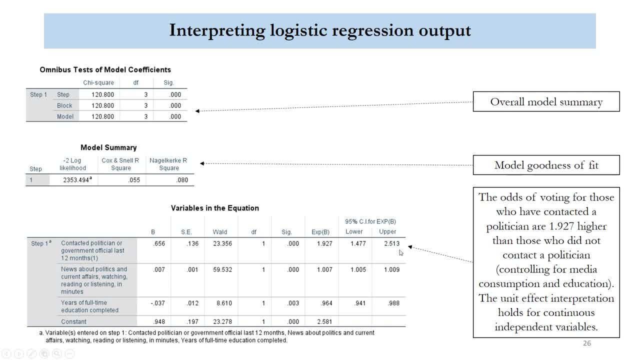 the reported odds ratio falls within the positive band here of the lower and upper bounds of the confidence interval. similarly, for this one we don't have a negative on the lower band and similarly for this one we don't have a positive on the upper band. this sort of this negative effect is within the range of the 95%. 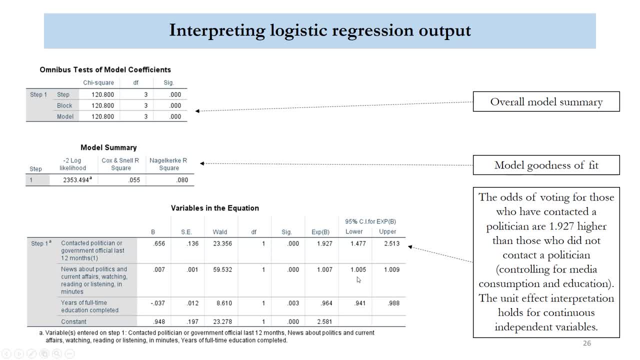 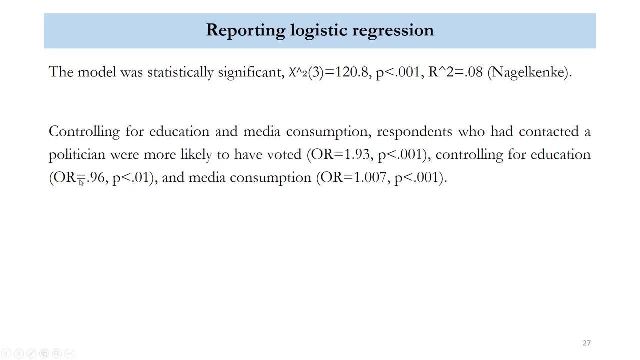 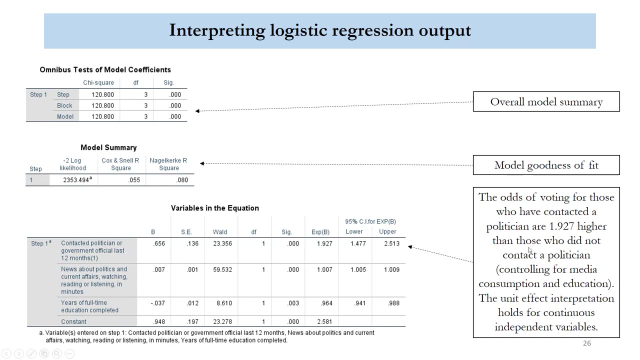 constant, but so we're reasonably sure that the effects of this one are negative, this one positive and this one positive, and you see our for each of these individually. we're simply reporting the odds ratio for each of our independent variables and we're reporting whether our they are positive or negative. so that's a good representation for the data type. so it's a good. 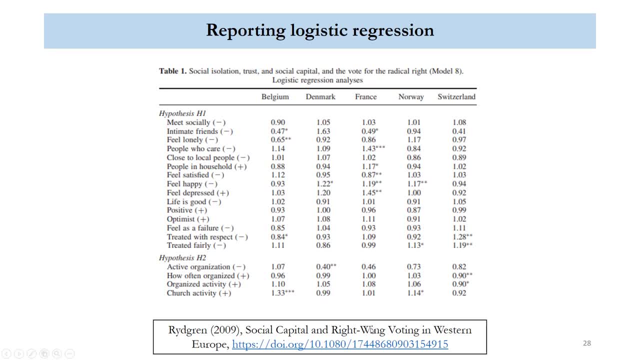 way of checking that the the values are positive. what's it like? so let's start with the data type, and we'll show you the data type in a moment, and then we're going to take a look at the data type at this point. so, for the data type, we're going to use the capital and the p value in the sig. 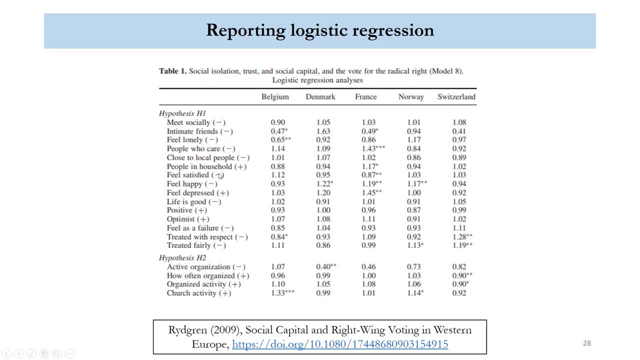 column falls below point zero, zero, zero. an example from the literature, then, is from the study of social capital and right-wing voting outcomes in western europe. so in this study the author has set up: life is good, this is the direction of coding, so positive, more depression and so on, so higher. 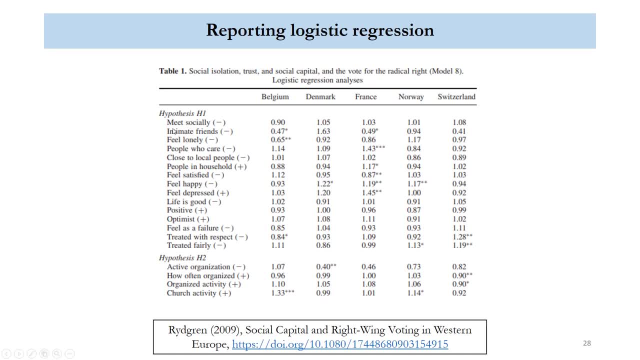 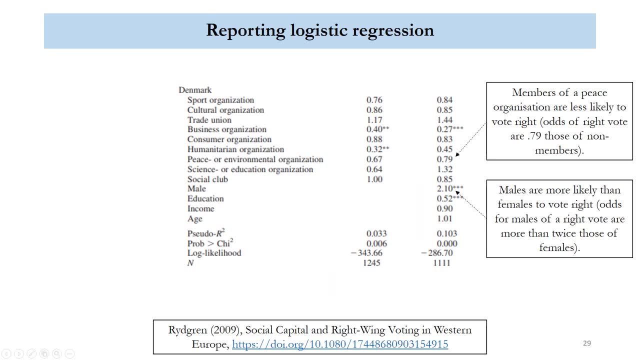 figures equal positive. um, these are different variables that measure different aspects of. i presume this is: yeah, this is measurement of social isolation. these are measurements of trust and in the model you see here, they test these different effects in a country context. so these are the results for denmark and they've got each of these little conditions here, whether or not someone's 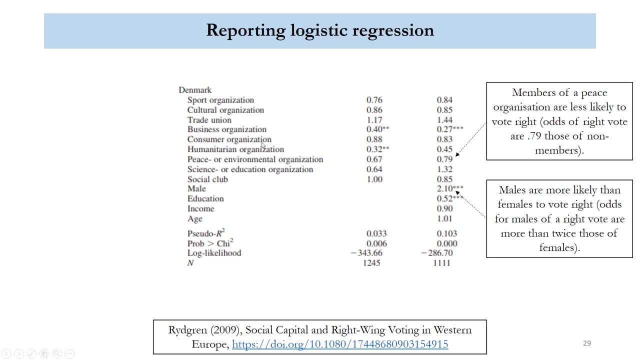 a member of a sport organization, cultural organization, trade union, business and so on- social club, whether they're male, their income units and their age in years. so if we take two of these, we see that these are the odds ratios: the odds ratio for members of a peace or environmental. 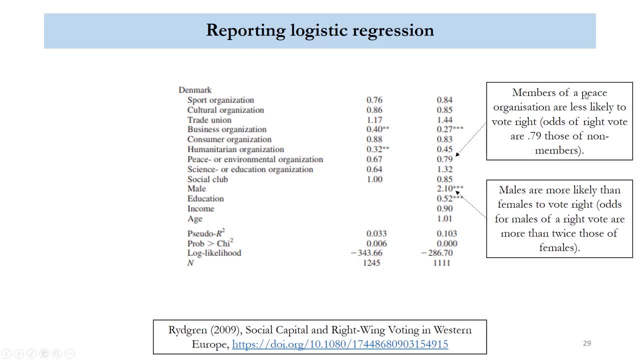 organization is 0.79. so we can say that members of a peace organization are less likely to vote right. the odds of a right-wing vote are 0.79, those of non-members. but males are more likely than females to vote, so the odds for males of a right-wing vote are more than twice those of females. so males are. 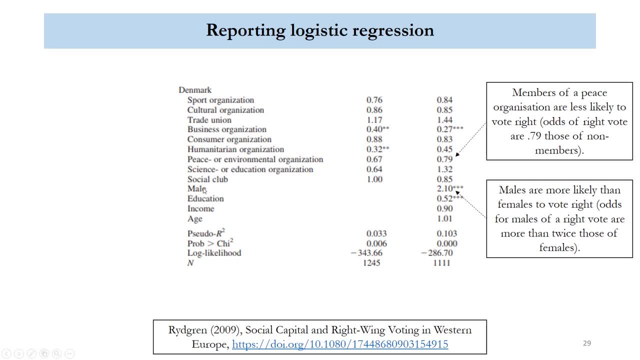 significant, more likely to vote right-wing than females. so, looking across all of these different conditions, using the odds ratios and using the p values, remember these little. you'll come across these little star indicators in the literature all the time. these are measurements, um of, of whether a um. 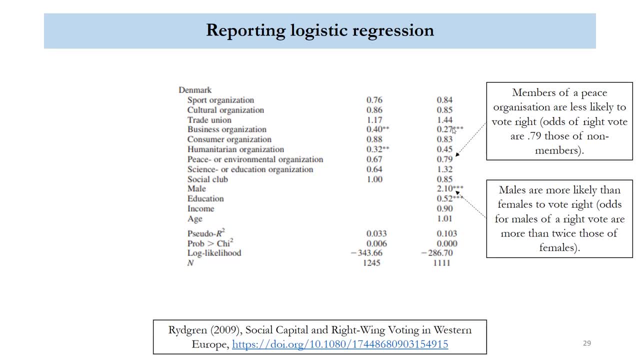 whether uh, the p value of a particular independent variable, has crossed a particular threshold of 0.05, 0.01 or 0.001. so significant effects here are whether an individual is a member of a business organization, whether they're a member of, whether they're male or what their level of education is. in this case, 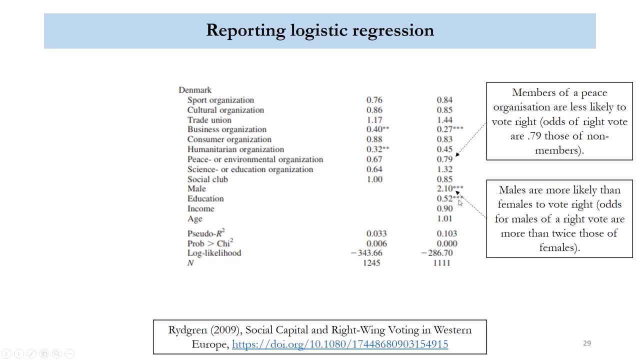 the more educated you are, the less likely you are, the less likely you are to vote right wing, and they've got their pseudo r-squareds here to compare across models. so we see here this model is doing a marginally better job because again we've got the inclusion of an additional block of independent 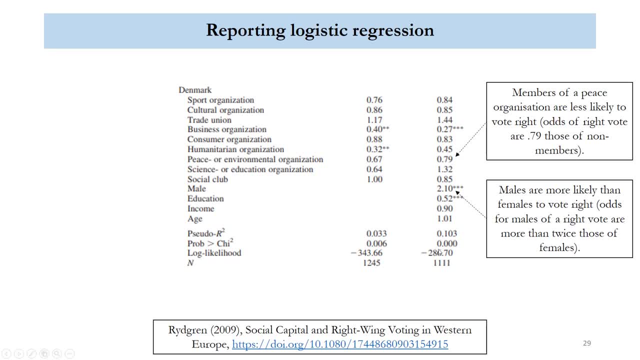 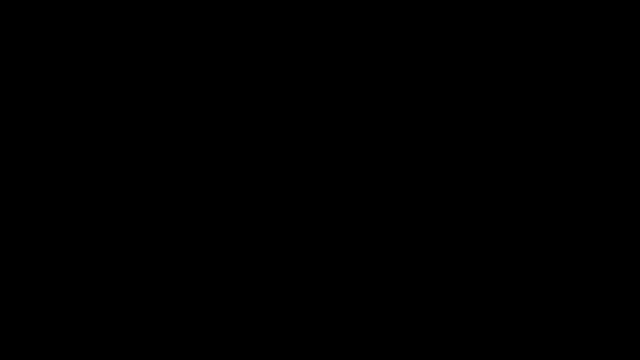 variables here as well. we've got our sample size and we've got the overall model significance for our chi-squared statistic as well. so we will look at some examples of this in class in week 12 on thursday. we'll look at the interpretation and we'll also look at how to set this up in spss.